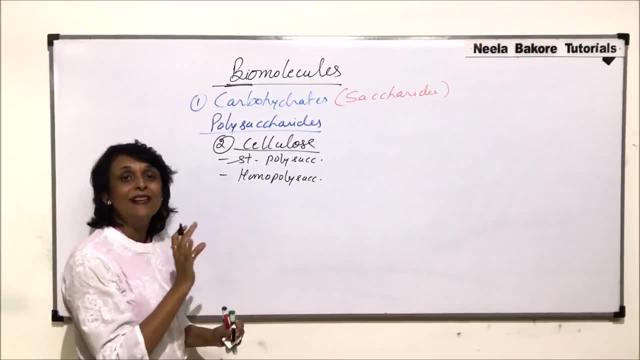 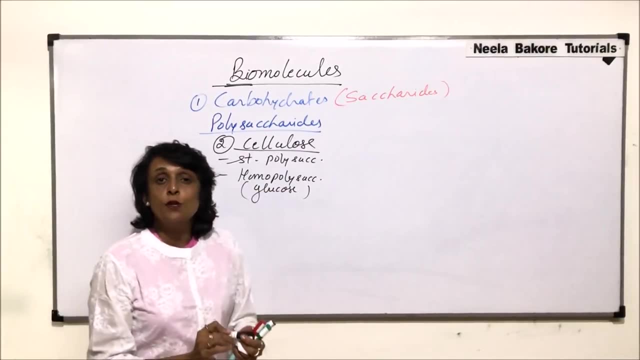 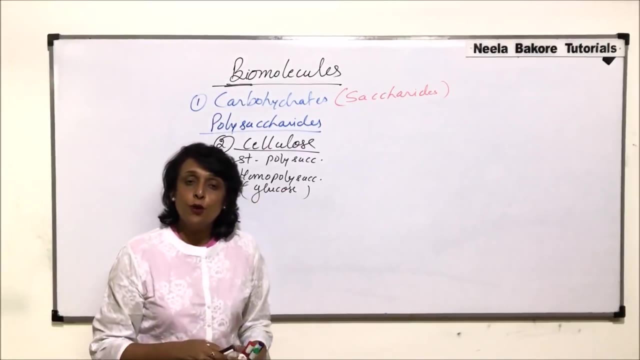 means it is made up of only one mono unit, That is, one type of mono unit, And that mono unit is glucose. So before this we talked about starch. Starch is also homopolysaccharide made up of only glucose, And cellulose is also homopolysaccharide made up of glucose. 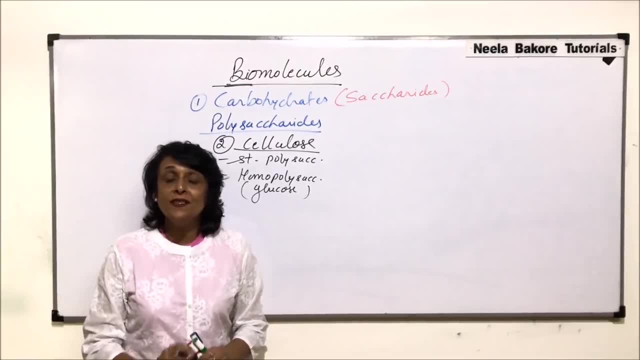 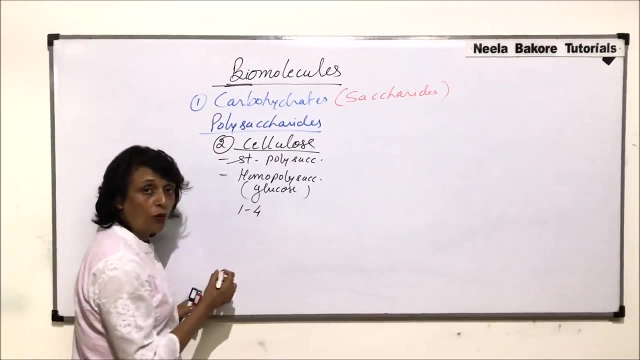 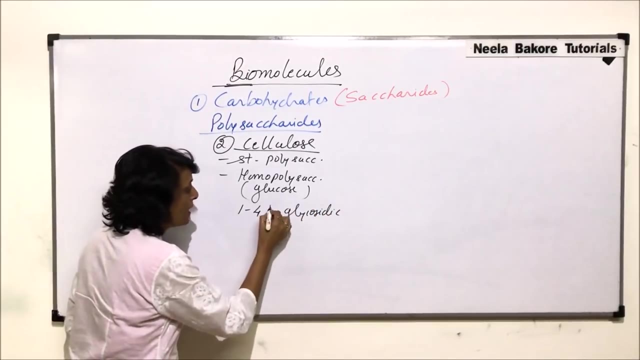 But there is a difference, And the difference is in the type of bond formation. Here the bond is 1,4-glycosidic bond, But the bond is 1,4, or we can write it here as beta 1,4-glycosidic. 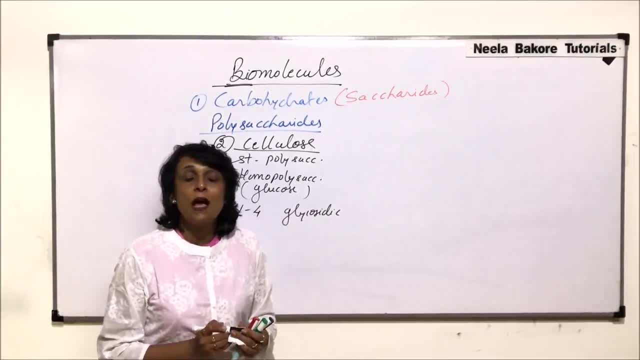 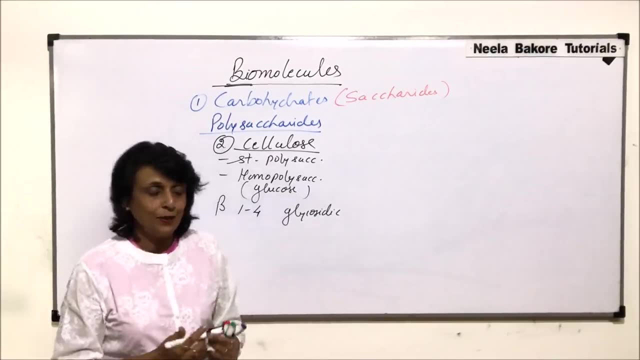 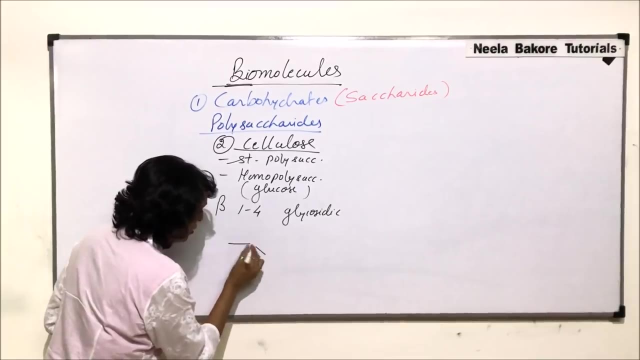 bond. That means glycosidic bonds are also of two types, And this is total glycosidic bonds And this is totally on the orientation of functional groups on the carbons. To understand it in a simple manner, suppose we make this glucose molecule the ring structure and we 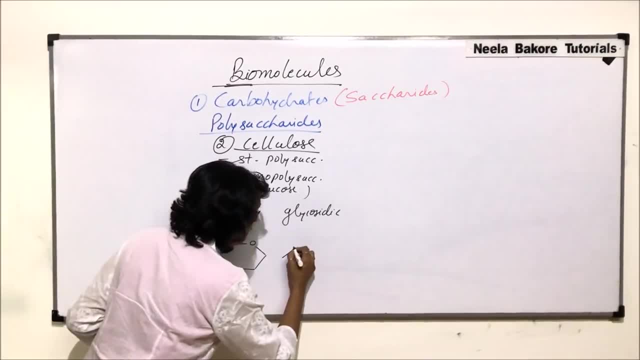 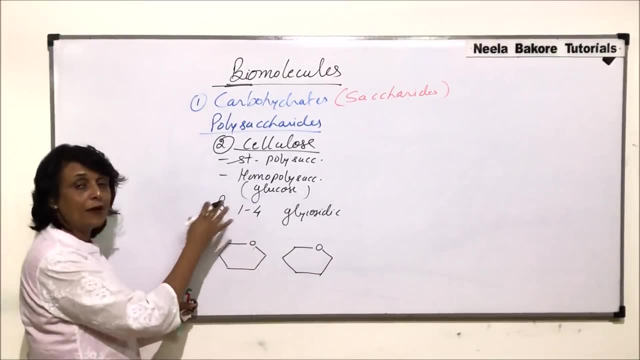 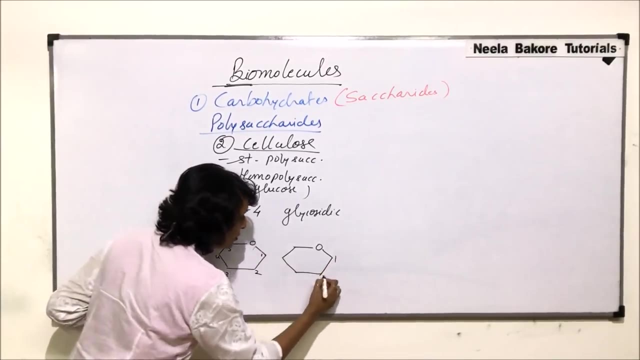 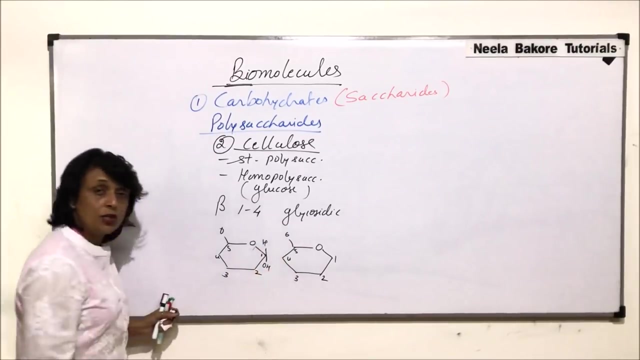 label the carbon numbers and see how the bond formation takes place. That will help us understand what is the difference between simple alpha, 1,4-glycosidic or beta, Say. this is carbon number- 1,2,3,4,5 and 6. Here also 5 and 6. In this case this is H and OH and here. 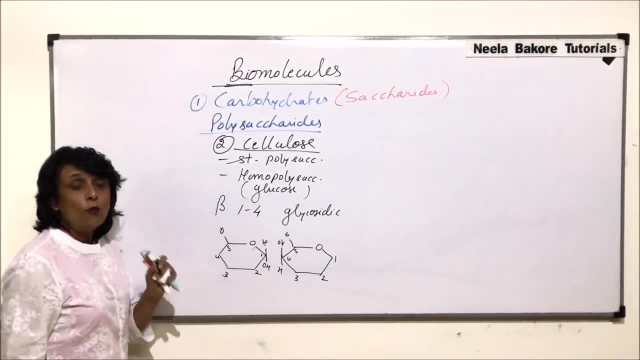 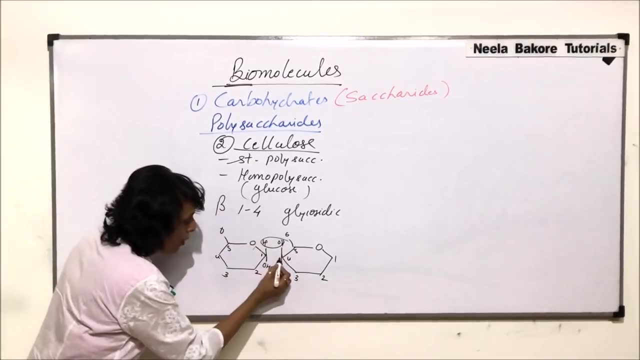 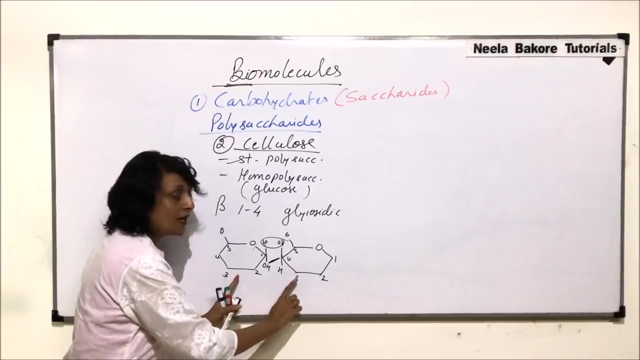 it is OH and H. Now when water molecule is lost, say, this is how the water molecule is lost. So the bond formation takes place in this manner: When the two glucose molecules which are making a bond, and the carbons between which the bond formation takes place, they do not have the same orientation of the functional group. The bond which is formed is called beta glycosidic bond. What difference does it make whether it is alpha glycosidic or beta glycosidic bond? For breaking a bond, we need a particular type of enzyme: The enzymes. 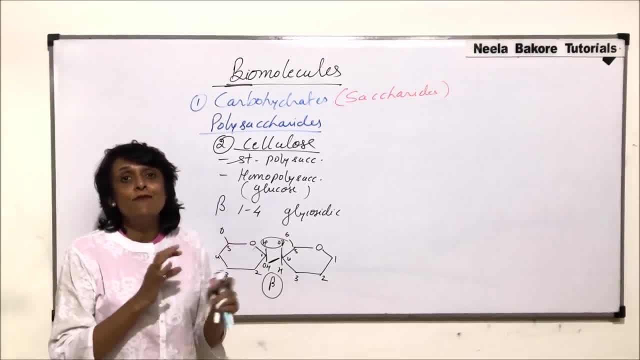 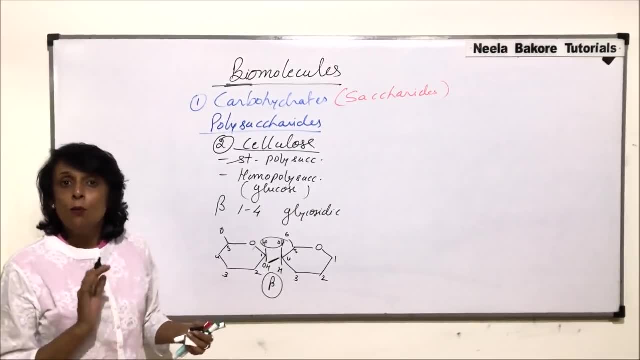 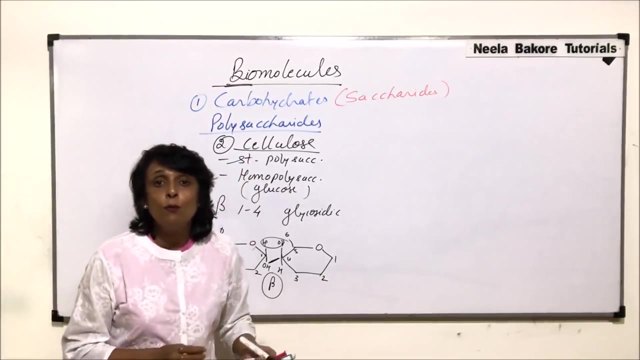 that we have in our body are called beta glycosidic bonds And beta glycosidic bonds. what we have in our body are all alpha enzymes. That means they can break only alpha glycosidic bonds. So beta glycosidic bond, which is present in cellulose, cannot be broken down by animals. 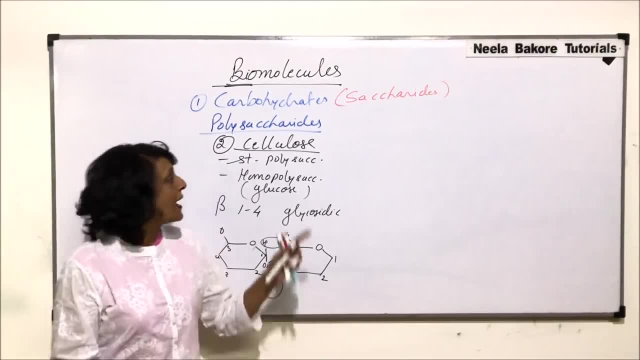 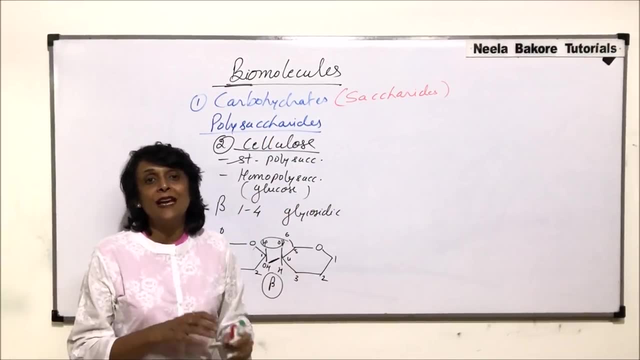 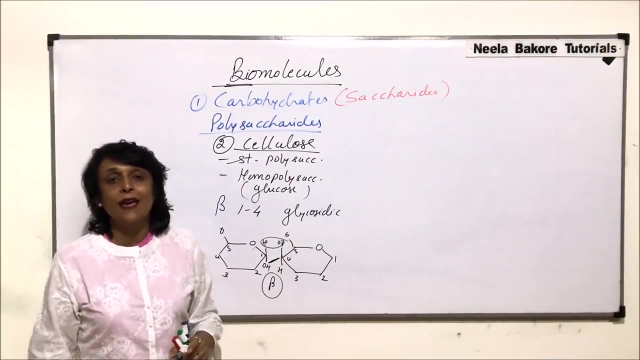 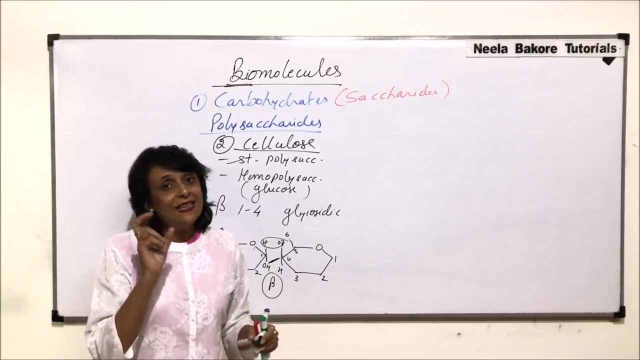 like us. Then how do some animals are able to digest this cellulose? This we have discussed in detail in the chapter of digestion, But quickly: animals like cows and buffaloes. they are able to digest cellulose because they have symbiotic bacteria in their stomach part and this bacteria produces an enzyme called. 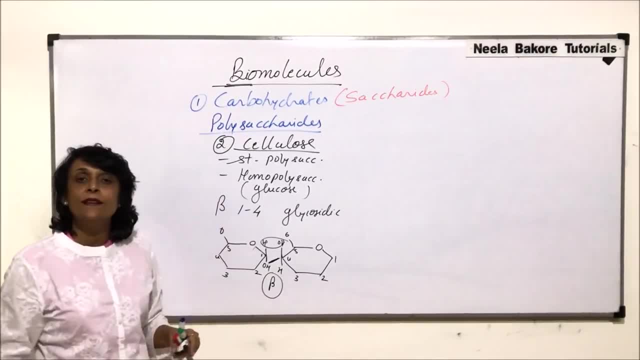 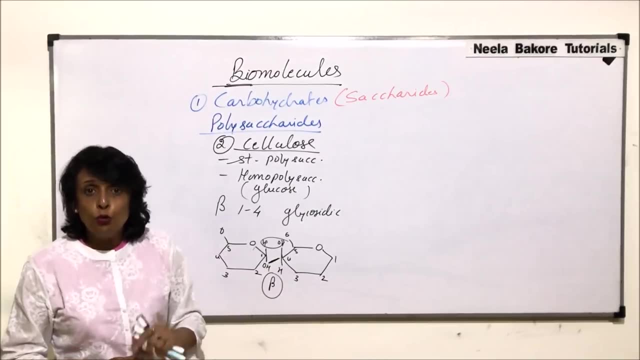 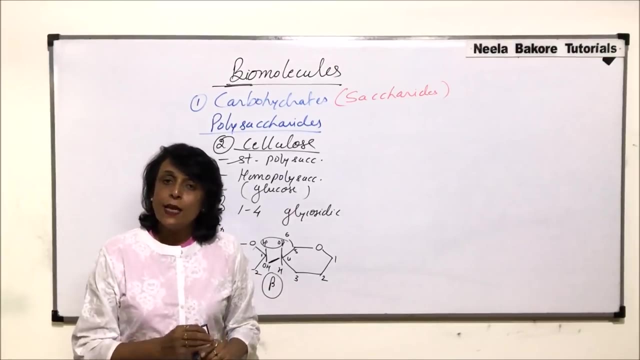 cellulase And this enzyme is capable of breaking this bond. So animals are not able to break this bond on their own. If some animals are able to do it, they are able to do it on their it, with the help of certain microbes like termites, can digest cellulose, but they have a protist which 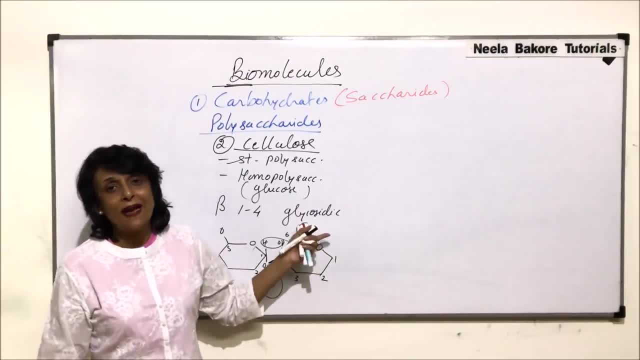 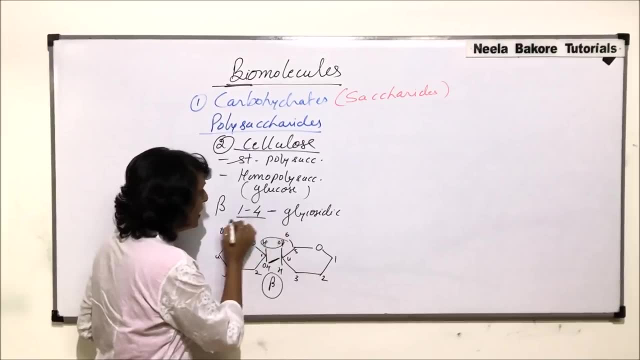 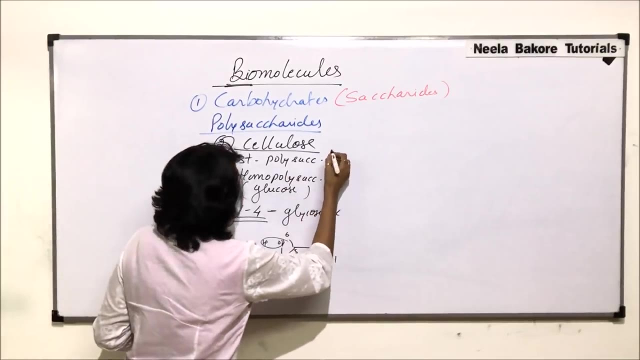 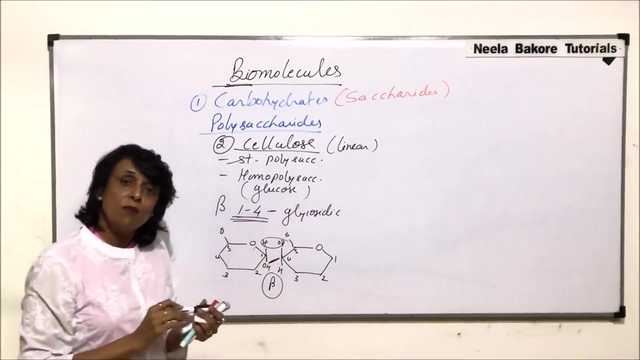 is called triconympha. cows, buffalos have a bacterium called ruminococcus, so they help in breakdown of this bond and it is only one full bond, that is. cellulose is also a linear molecule. so cellulose is a polysaccharide which is linear, and the reason for its linear nature is because it. 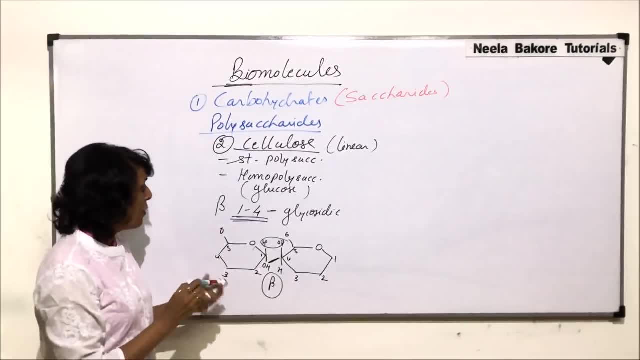 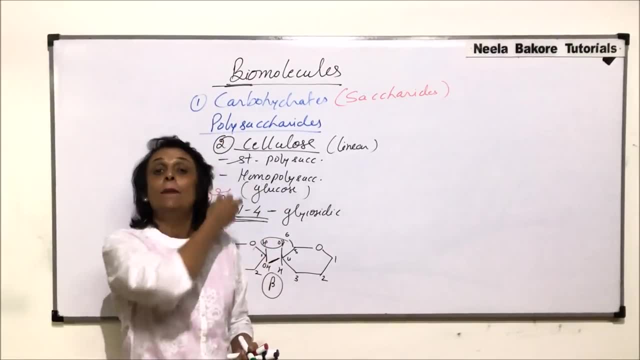 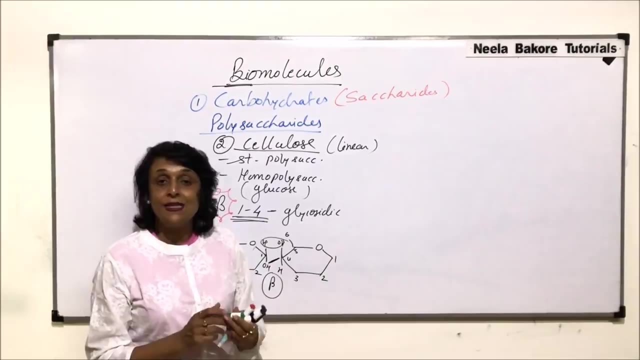 has only one four bonds, but the one four bond is a beta bond, and to break a beta bond we need beta amylase, which we cannot synthesize. so cellulose again, another very important polysaccharide. it is helping in formation of cellulose well. other than that, where else is cellulose present and can we use it in some other ways? 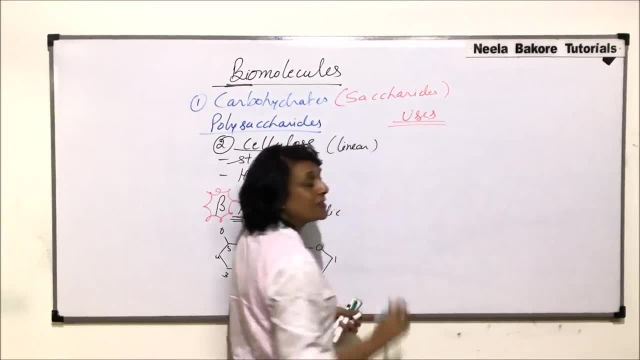 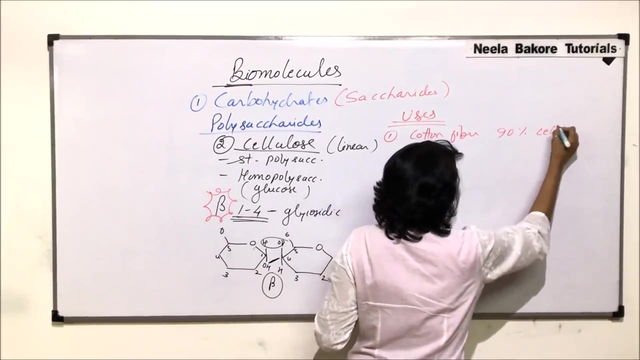 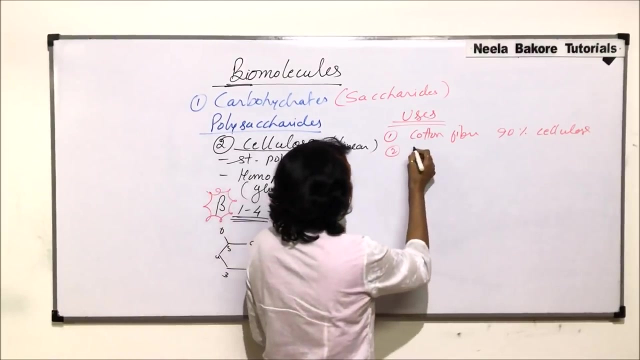 so if we have to sum up uses of cellulose, we can list out few important things. cotton fiber is actually 90 percent, or more than 90 percent, cellulose. so 90 percent is cellulose in case of cotton fibers, not only cotton, other fibers, these fibers like jute, 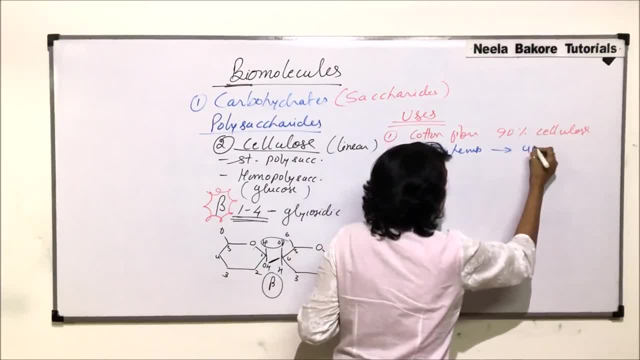 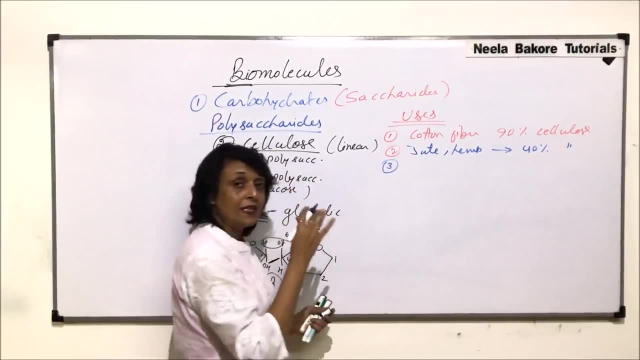 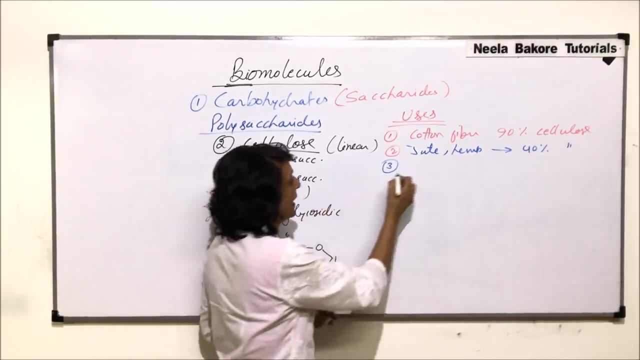 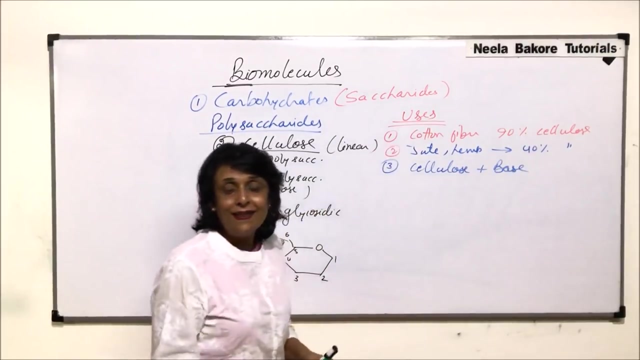 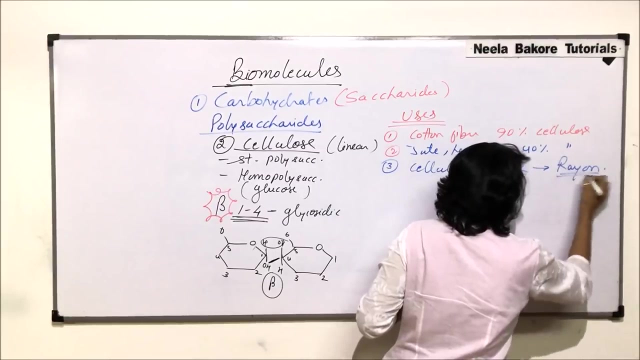 hemp. they also have 40 or more percent of cellulose. few chemical variations. that means if we dissolve cellulose into something or we make it react with something that also can be used. for example, cellulose when dissolved in a base, or alkali which is formed, is used to make rayon, and this rayon is known as a synthetic fiber. 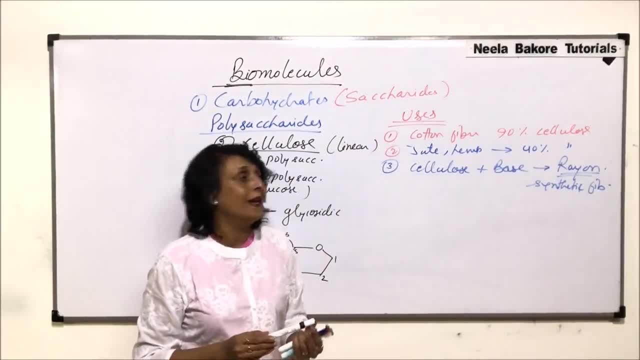 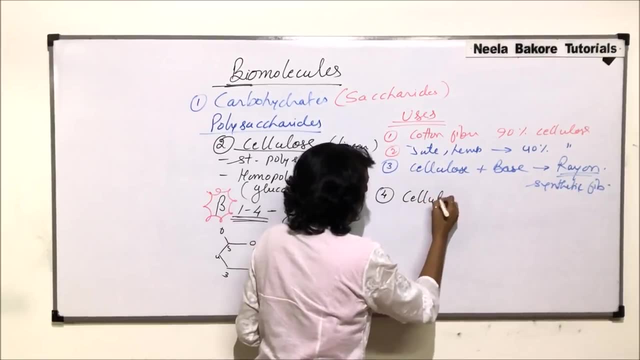 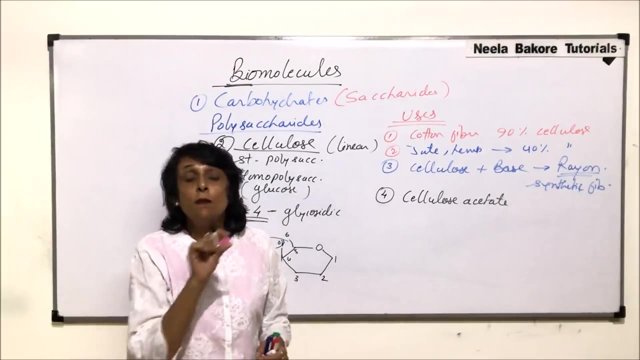 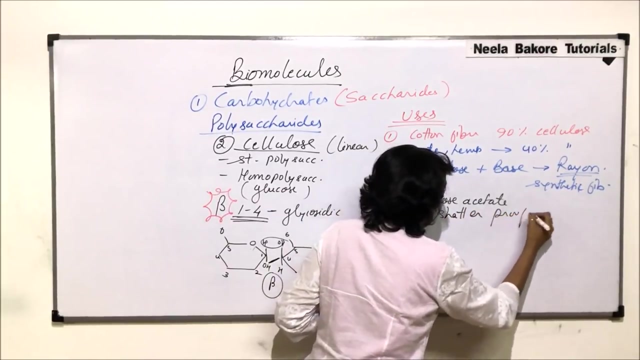 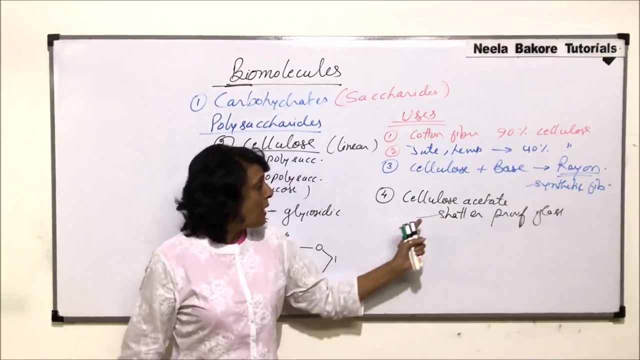 so this rayon which is obtained is also obtained by dissolving cellulose into an alkali. next modification is cellulose acetate. cellulose acetate is used to make films and shatter proof glass- shattered proof glass. nowadays, the windshields of automobiles are made out of. 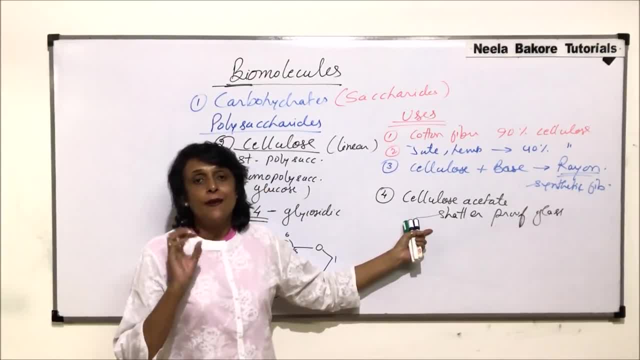 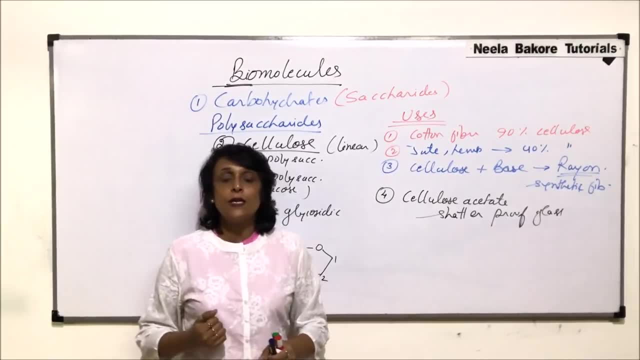 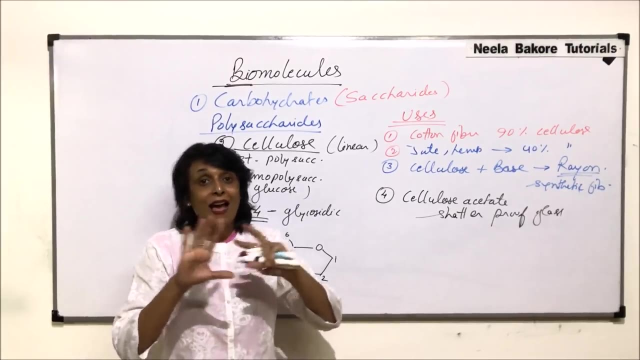 the shatter proof glass. very simple to understand: when something hits a normal glass, the glass breaks and its pieces fall off. but nowadays, when we see a car and suppose it has hit by a stone or there was an accident, the glass breaks but the pieces don't fall. 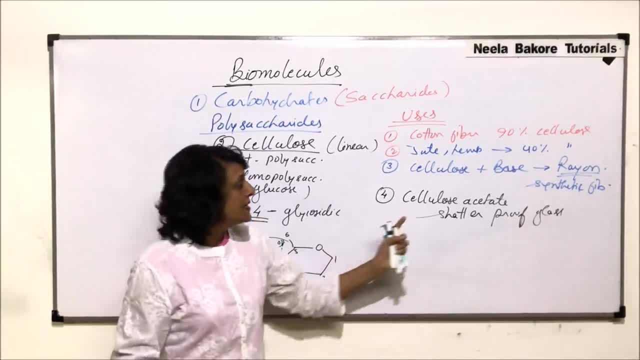 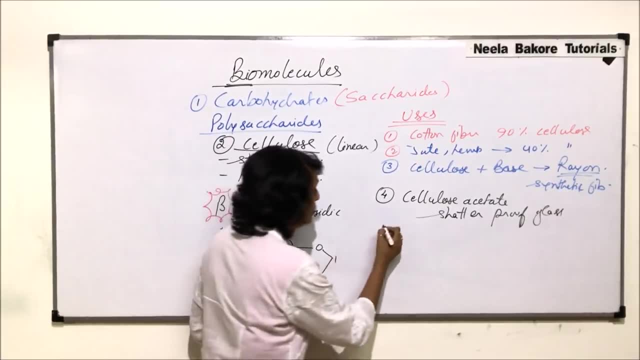 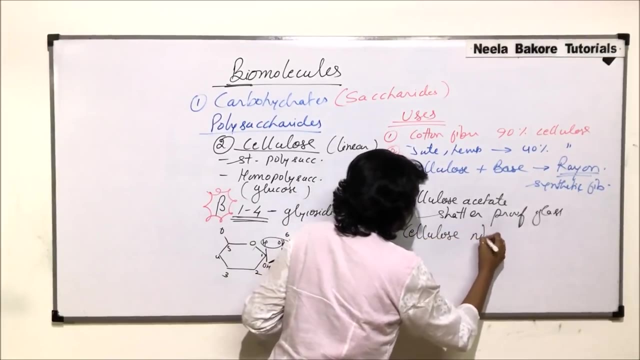 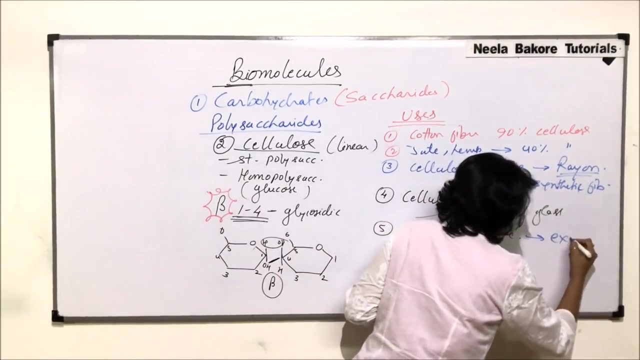 off, they remain in that layer itself. such a glass is known as shatter proof glass, and cellulose acetate is used to make such kind of glass. another chemical variation is cellulose nitrate. cellulose nitrate is used to make explosives- one more use of cellulose. 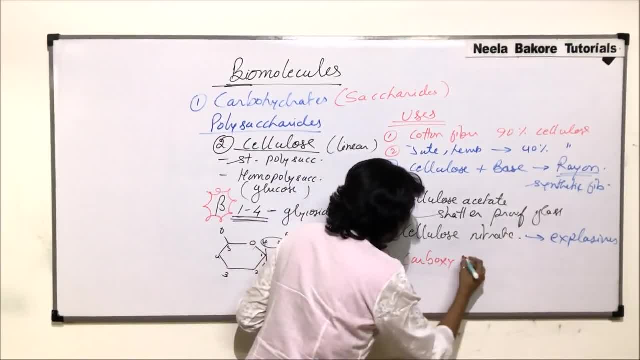 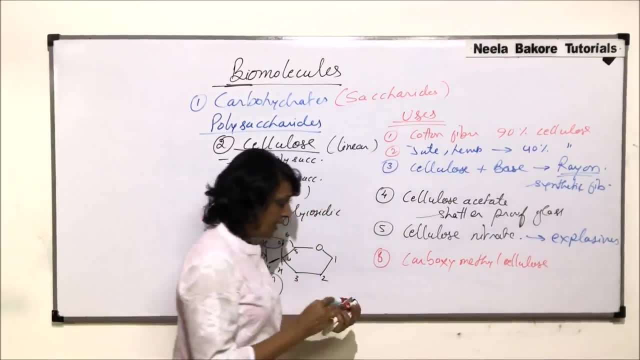 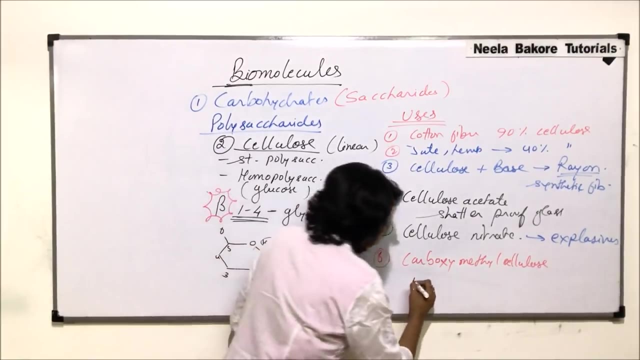 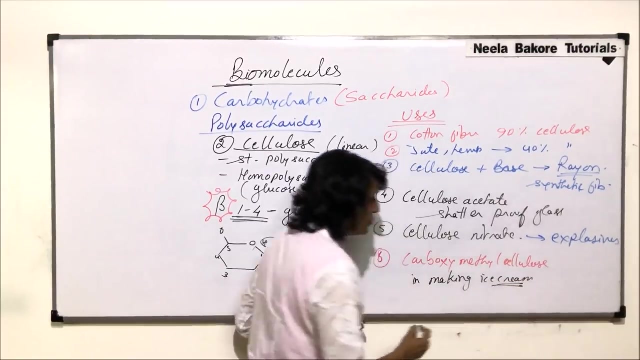 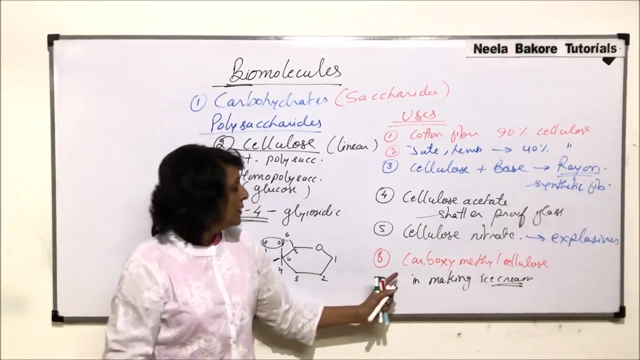 it is carboxymethyl cellulose. carboxymethyl cellulose normally used in making ice creams in making ice creams and reason why it is used in making ice cream, because it provides smoothness. in many ointment also, this carboxymethyl cellulose is used to provide that smoothness or the